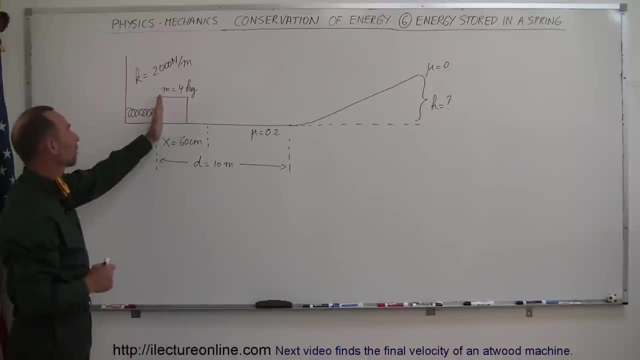 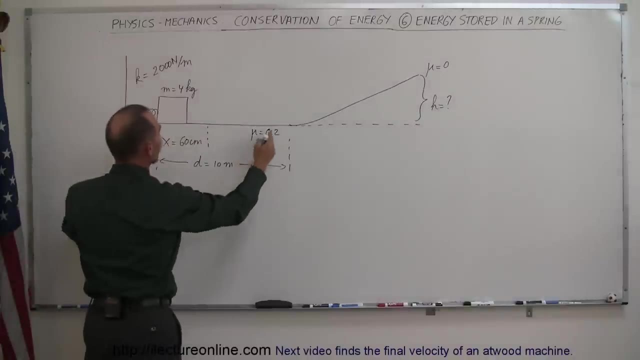 which is being compressed a distance of 60 centimeters. The object placed in front of it has a mass of four kilograms. The block is released. The block starts sliding forward. It has to overcome a distance of 10 meters along the horizontal path, with a friction of 0.2 meters. 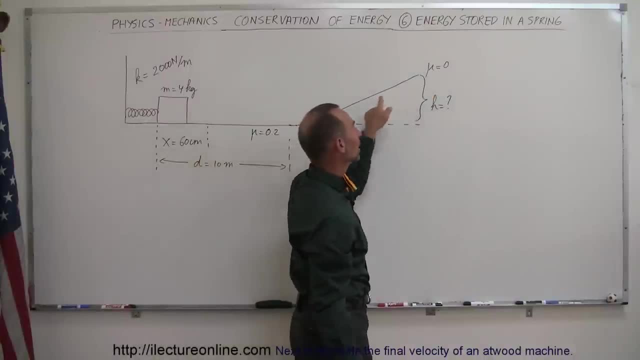 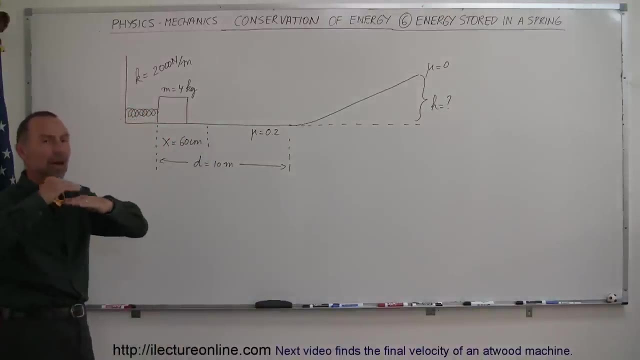 Then it hits the incline. At that point there's no longer any friction on the incline And the question is: how high will it reach along the incline? So not how far along the incline, but how much height will it gain before coming to a stop. So, again, the only thing you have to worry. 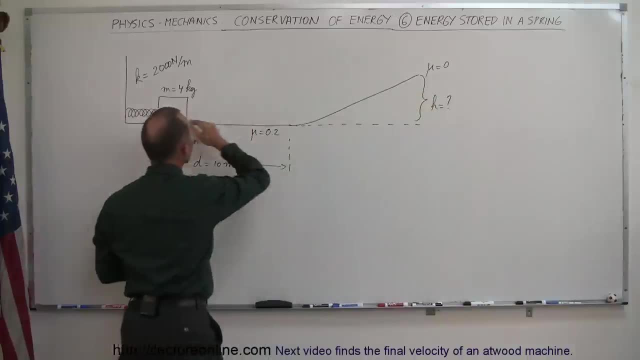 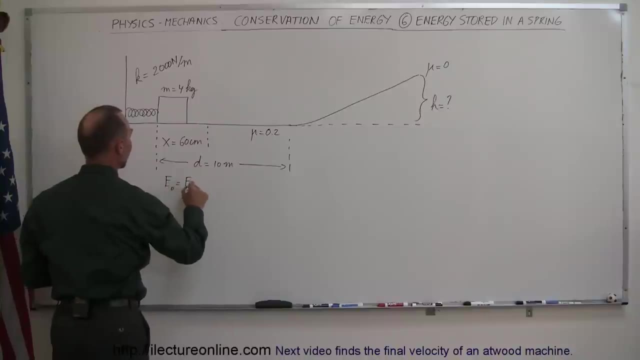 about is the initial state, the final state and any friction loss throughout the process. And of course, we're going to use the equation energy initial equals energy final, or any work put into the system plus any initial process. Potential energy plus any initial kinetic energy is equal to any final potential energy plus any 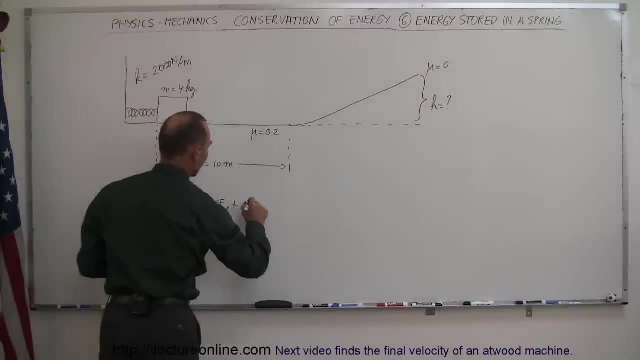 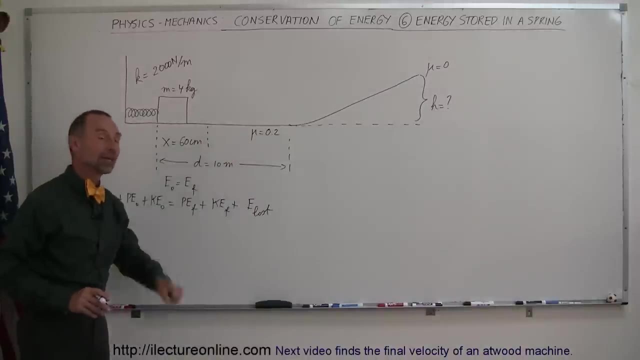 final: kinetic energy, plus any heat loss or energy loss due to overcoming friction or wind resistance and so forth. We have friction, so definitely there will be something lost right here. All right work put into the system, that is equal to zero, because we are not pushing the block while it's. 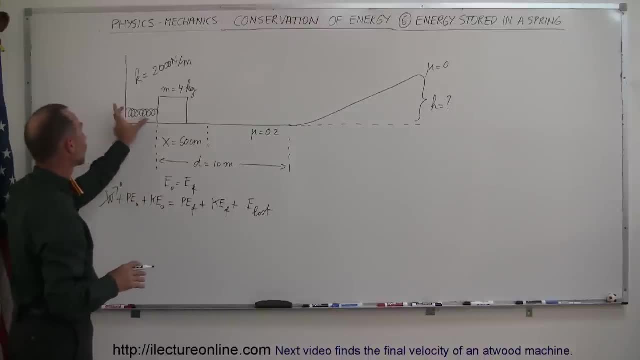 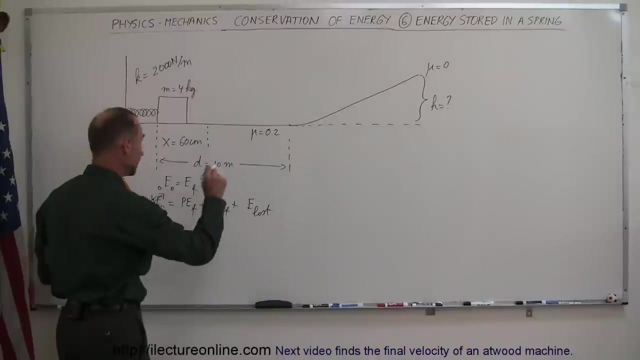 moving. Potential energy initial: yes, we have that because there's a compressed spring right here. so we have one half k x squared Kinetic energy initial: we have none because it's not moving at that potential, at that point. Potential energy final: we do have because we have gain height. 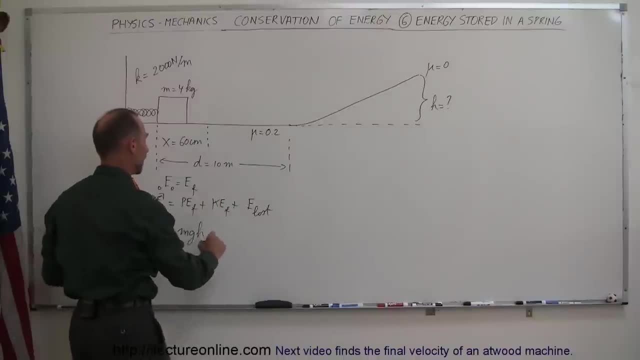 so it'll be m, g, h. Kinetic energy final would be zero because it's not moving at the very end when it reaches its maximum height and energy lost will be there. It's plus the friction force times the distance along that path where there's friction. 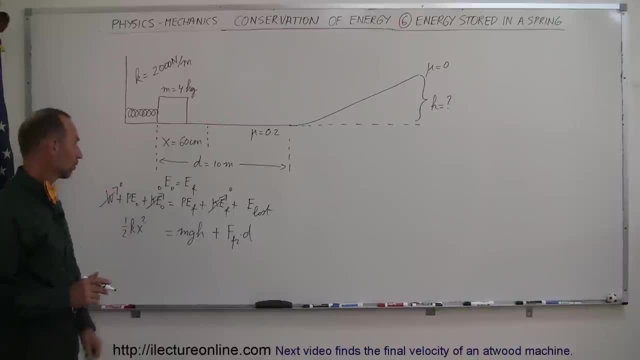 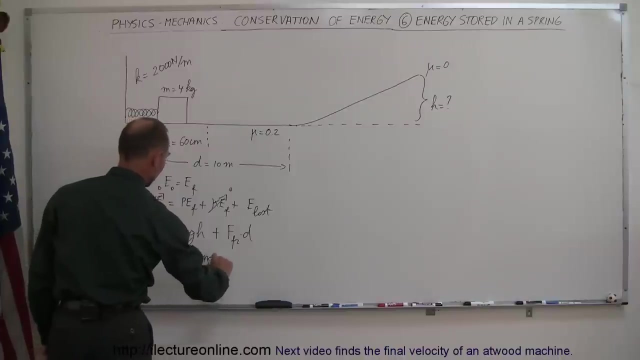 What are we looking for? We're looking for h, so we have to solve this equation for h. We can go ahead and do that by moving this over to the other side. So we have one half k. x squared minus force, friction times, distance equals m, g, h. Now, if you look at it like this, notice any energy that was. 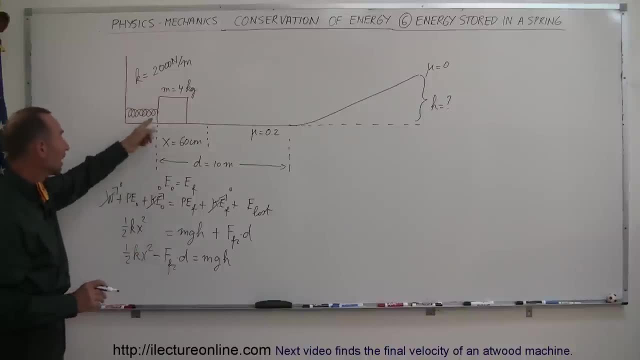 stored in the spring, which will be given to the block, minus the energy required to overcome the friction, will equal the final potential energy. So we have k x squared minus force, friction times, mu. So that makes a lot of sense when you look at it like that. We're now going to divide both. 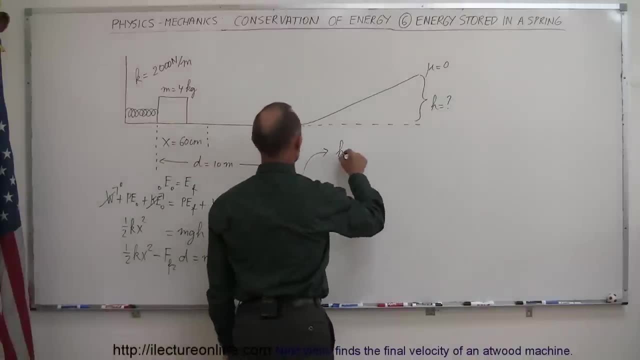 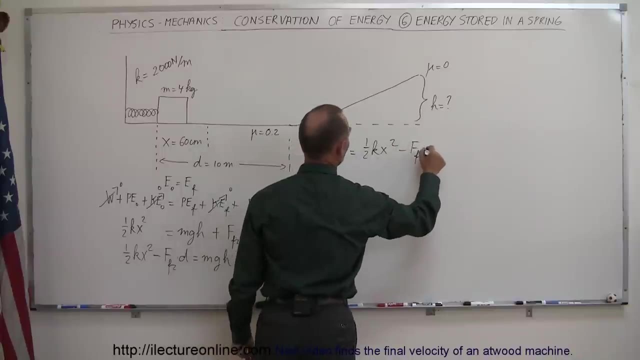 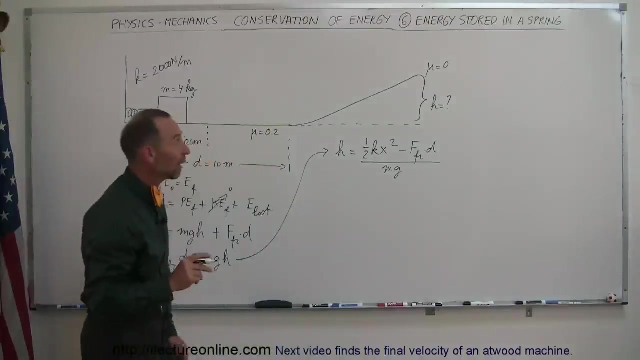 sides by m- g. so we can then say that h is equal to the left side of the equation, which is one half k x squared minus force, friction times distance divided by the coefficients of h, which is m times g. Now the only thing left to do here is find out what the friction force is equal to. 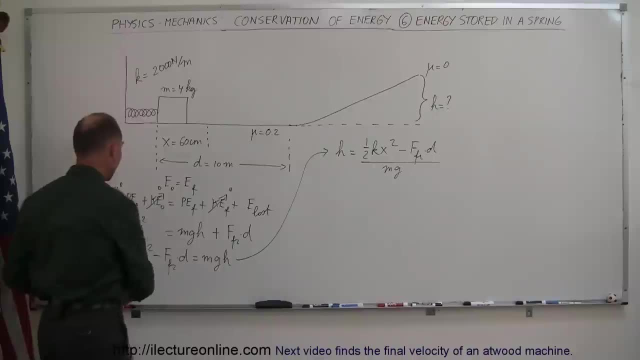 which is equal to the weight of the object. times mu. Remember that we have the weight of the object because of gravity. we have the normal force, which is equal to that weight in magnitude because it's on a flat surface. So n is equal to mg, just in the opposite direction. 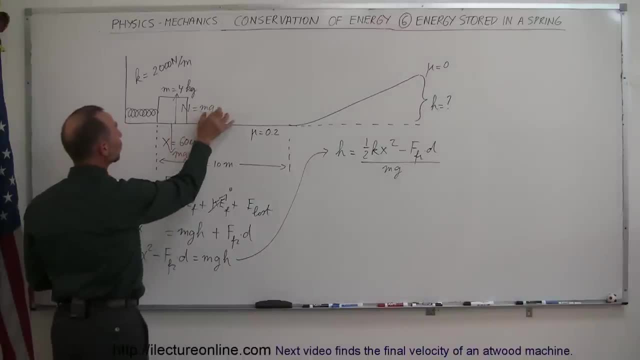 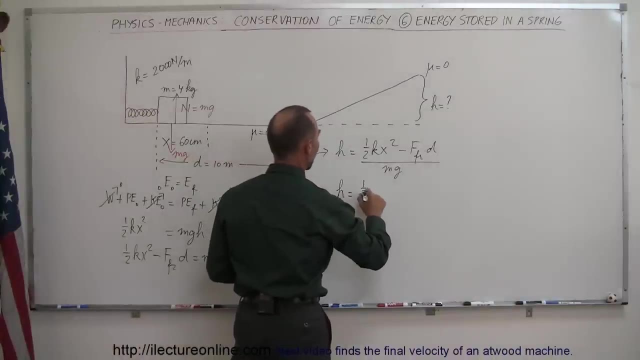 and then of course for the friction force we take it n times mu or mg mu. so when we plug that in here we get the height gain is equal to one half k x squared minus the normal force, which is mg times mu times d, all divided by mg. 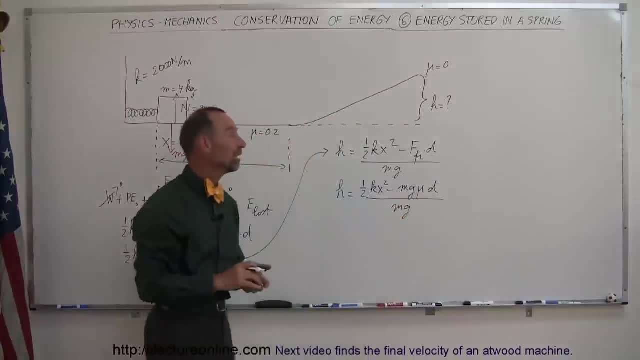 if this term is bigger than this, of course it doesn't even make it to the incline that will stop prior to making that incline. that could happen, we don't know for sure. if all the energy is lost before it makes the incline, of course h will be zero, and then the question may be how far 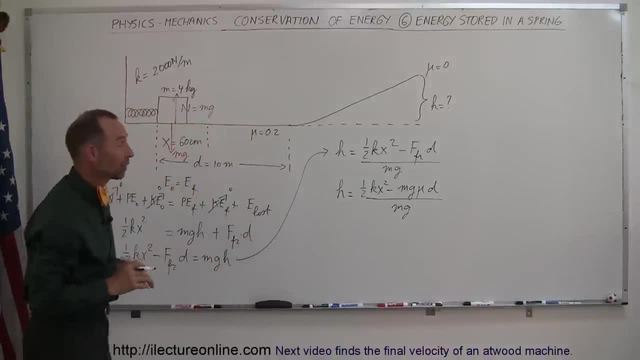 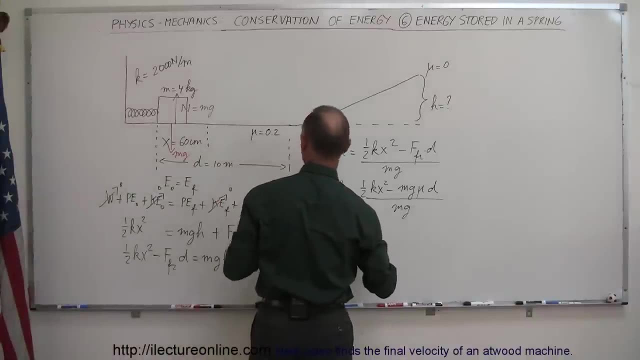 along this, this horizontal pad, does it go, before coming to a complete stop? so let's find out what that's equal to. so this is equal to one half times k- i'll leave the units off, make it cleaner. 2000 times x, squared, which is 0.6 squared, minus the mass, which is 4 g, 9.8 mu was equal to 0.2. 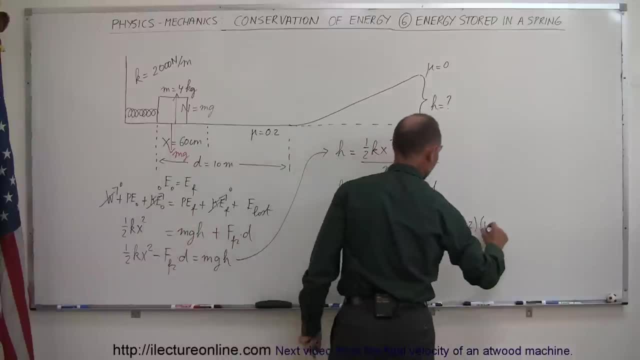 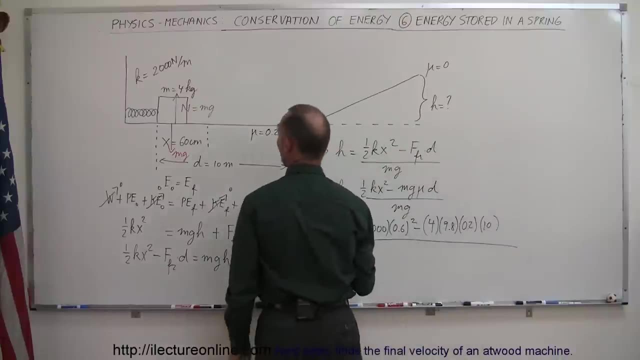 right here and the distance was 10 meters. so this is the energy lost by overcoming friction. that's how much energy was stored in the spring, and if we divide that by the weight of the object, which is 4 kilograms times 9.6, that will tell us how high it managed to go.